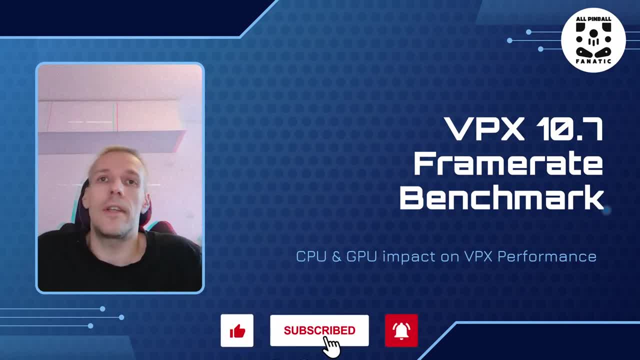 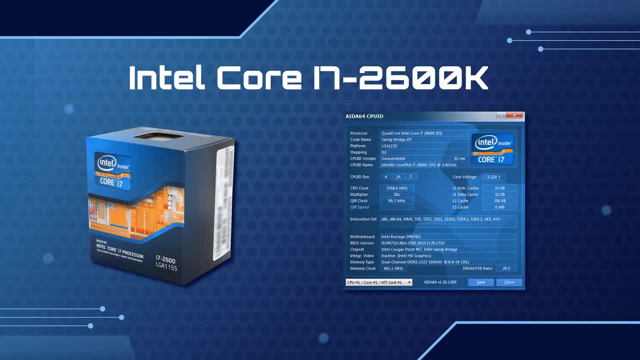 don't forget to subscribe to the channel, which will motivate me to record more stuff, and hit the notification bell to receive info about incoming videos. I play on my virtual cabinet at 4K resolution with 60Hz refresh rate using a LG TV screen and. 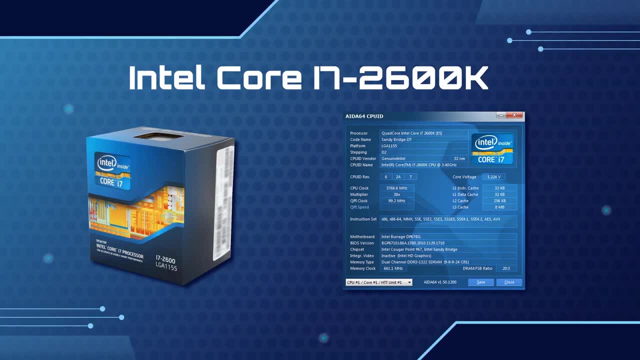 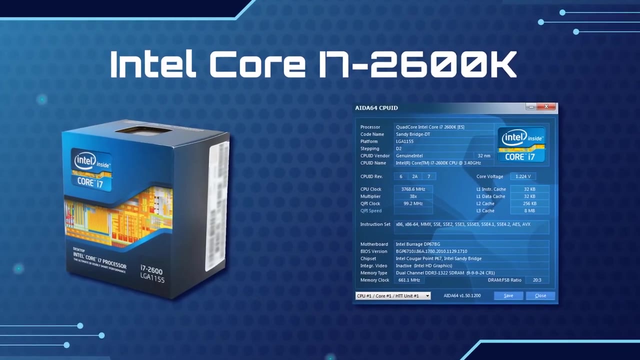 my system specs were Intel Core i7 2600K locked to 4 GHz, plus 16 GB of RAM and GTX 1070 graphics card. for some time since I built my cabinet, The amount of RAM is not so important for the benchmark, so I won't talk about it. 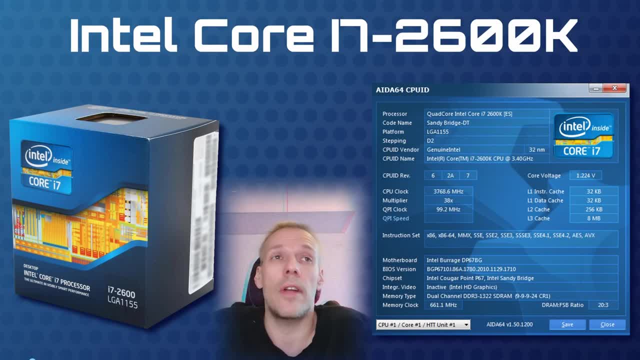 The GTX 1070 graphics card wasn't quite enough to get the stutter-free action on all of the tables, especially the newer ones from the VPN Workshop team or Flipper, which are beautiful but heavy performance-wise. So, after reading here and there, mostly on the VPX-related forums and Facebook groups, 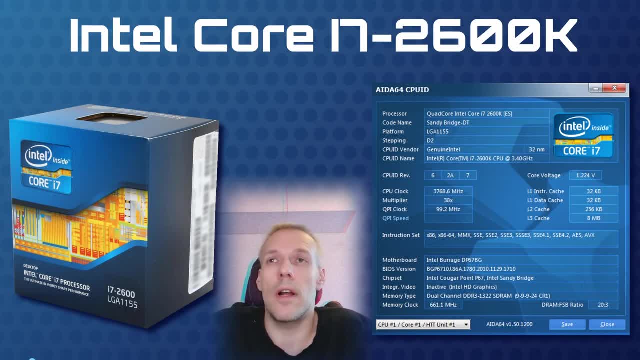 I came to conclusion that I need to get a faster graphics card, So I bought, used GTX 1080 and it was better with it, but only a bit and not that much as I would expect, so started to dig deeper. My CPU was a bit old, released around 2012.. 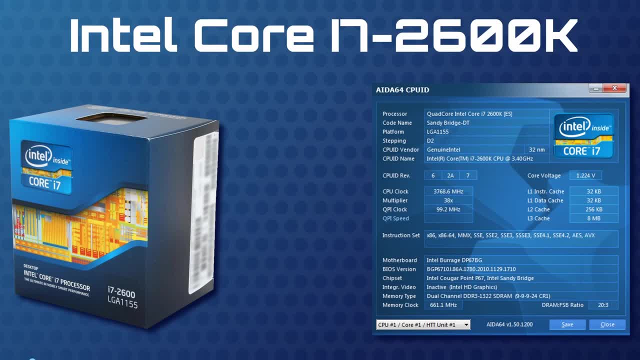 It was good enough for the VPX, as many claimed that my only problem was the graphics card, So I thought that I will swap the GTX 1080 card with the one I have in PC I work on – RTX 2070 Super, and I will have all my stuttering problems gone. 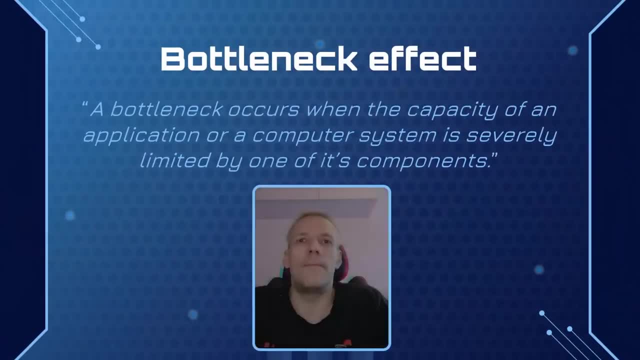 I wish I knew that. it was far from being true. There is something called a bottleneck effect. The speed of an application or a computer system is severely limited by one of its components. So if all of the components of a PC are not able to fit the same amount of data at the 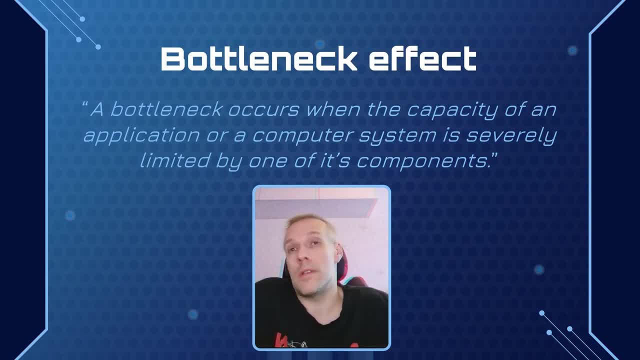 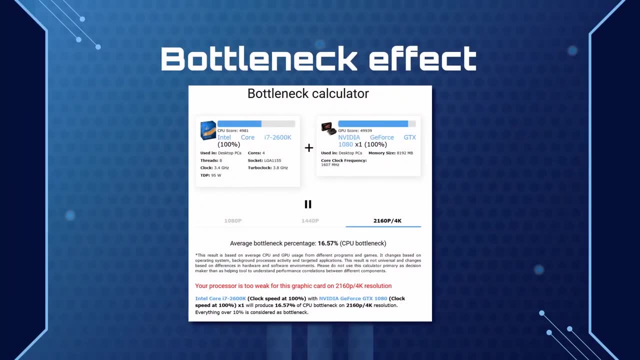 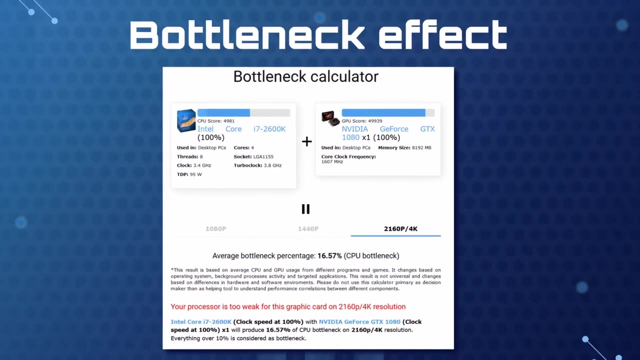 same speed, a delay is created. so system performance is defined by its slowest component, not the fastest. So I have used one of many bottleneck online calculators and that's what I got: The i7-2600.. It's a very good computer. 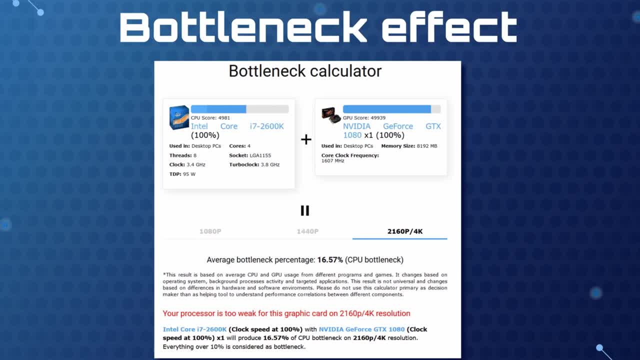 The 600K CPU paired with the graphics card I have, the GTX 1080,, gives a bottleneck of over 16% at 4K resolution. The calculator clearly states that your processor is too weak for this graphic card on 4K resolution. 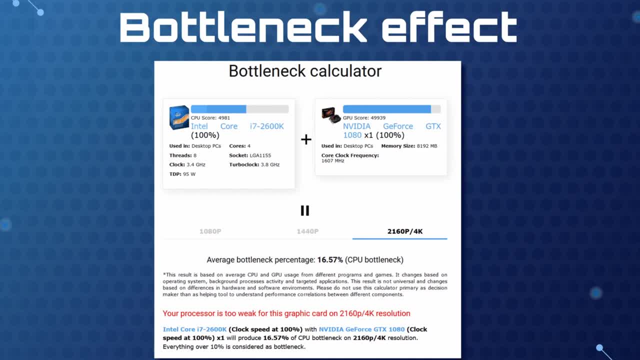 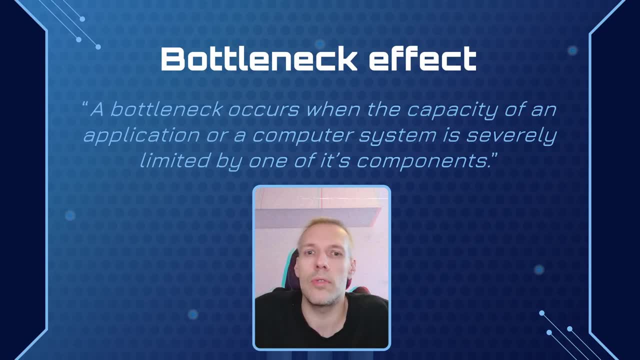 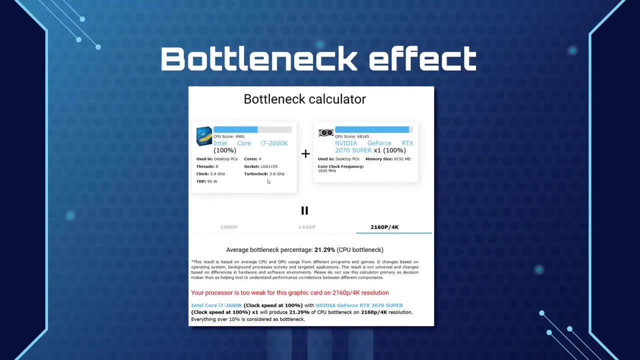 which means that graphic card is not using its full potential. So I started to think: If I swap the graphic card to a better one, the mentioned RTX 2070. The bottleneck would be even worse, or not? So I checked it in the calculator. 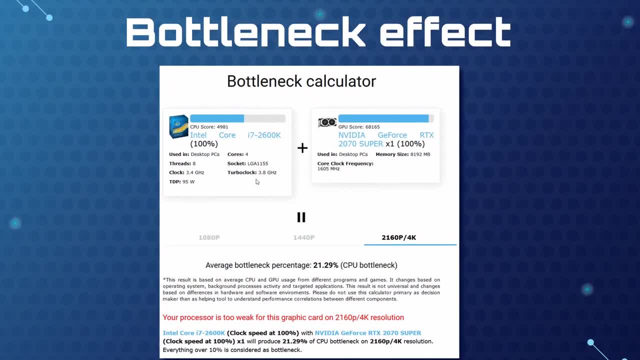 And indeed a bottleneck of over 21%. So that would be a lot of wasted computing power of that card too. So I started to think about upgrading my CPU, which unfortunately is connected to replacing the motherboard and memory chips, because it's already 11 years old configuration. 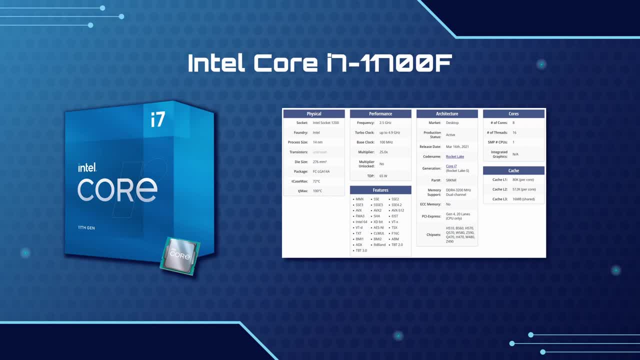 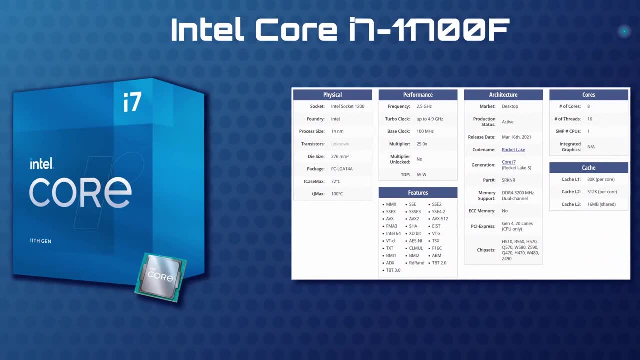 I chose Intel Core i7-1170.. It's a very good CPU. I got the i7-700F, the 11th gen processor. The F means that it doesn't have a built-in graphics card chip and the frequency clock. 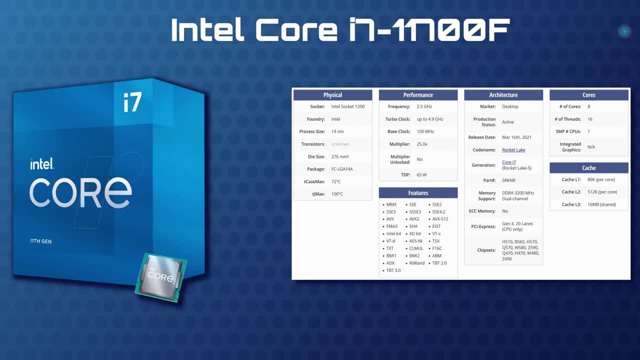 is not unlocked so it's not that easy or safe to overclock it. I was fine with no OC possibility because I don't like to overclock and found it cheaper than K and KF. Checked the processor in bottleneck calculator With the GTX 1080 card. 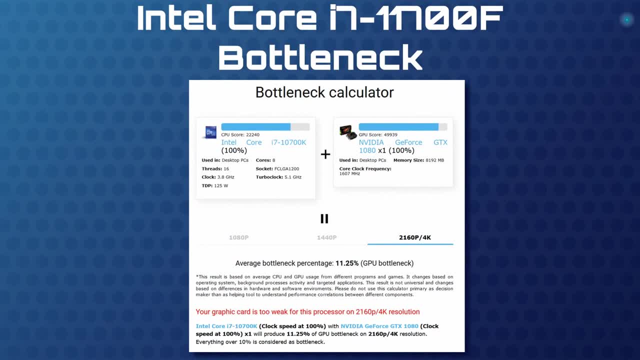 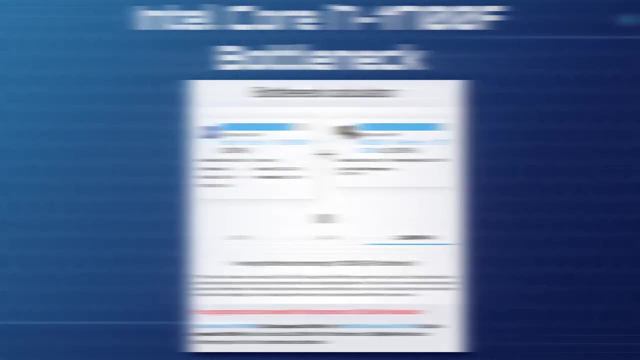 And it turned out that for this system the graphic card is too weak, but only a bit. All over 10% is considered bottleneck. So according to this, with this CPU the GFX card would run at its full potential, but CPU would not. 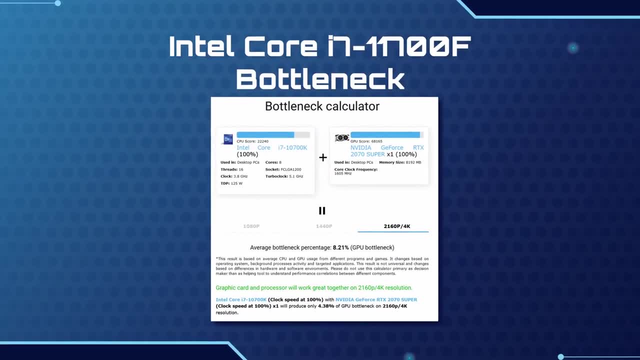 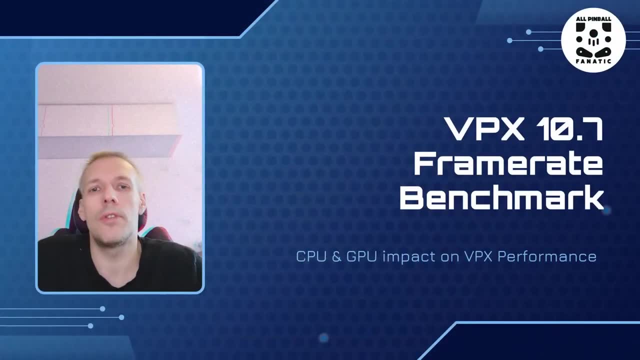 So I checked the RTX 2070 super card and finally I got the green check saying that these two would perform great. After all this, I came to the first important conclusion, For VPX: CPU is important as much as the graphics card is. 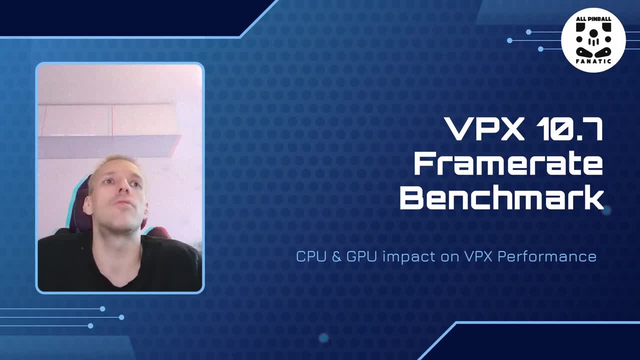 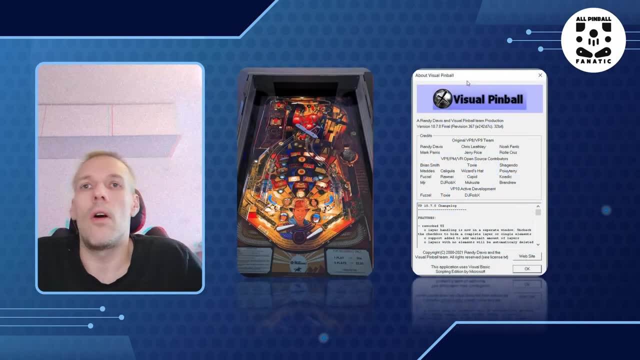 But what's really the impact on the most important thing in playing virtual pinball, The framelane? I decided to check that doing the following benchmark Whole test is performed on the final version of the VPX 10.7, Revision 367 using IndianaJones. 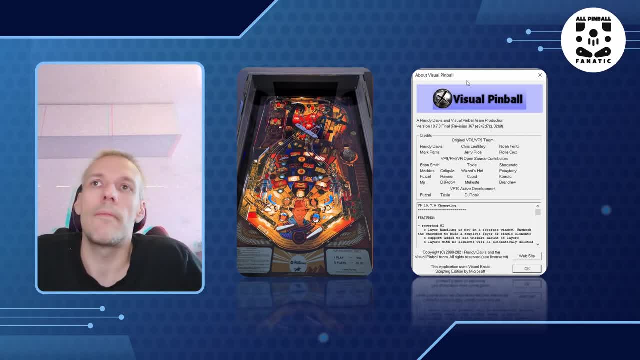 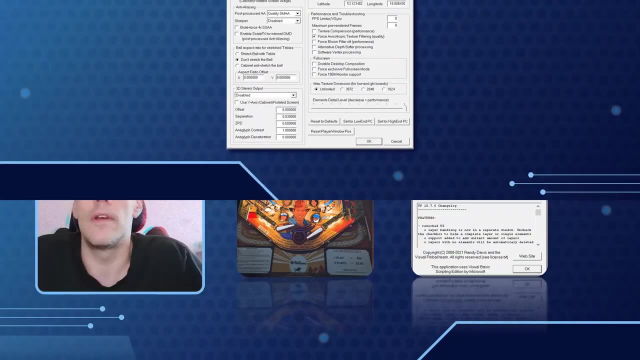 the pinball controller And the pinball adventure table from VPN Workshop. First, I selected four configuration of VPX video graphic options that I have been fiddling with to get better framerate when playing tables, starting with performance hungry one First configuration is all buzz and whistles. 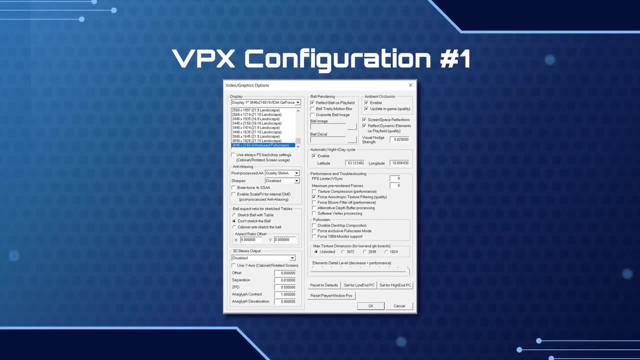 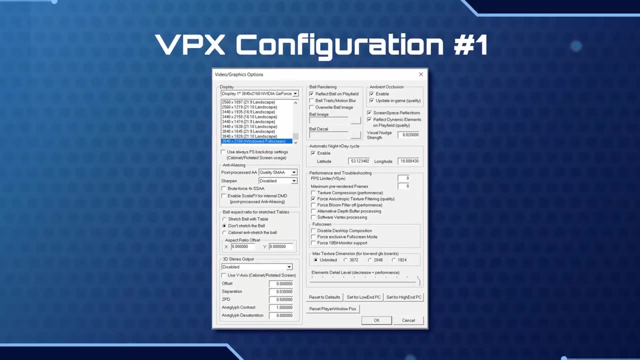 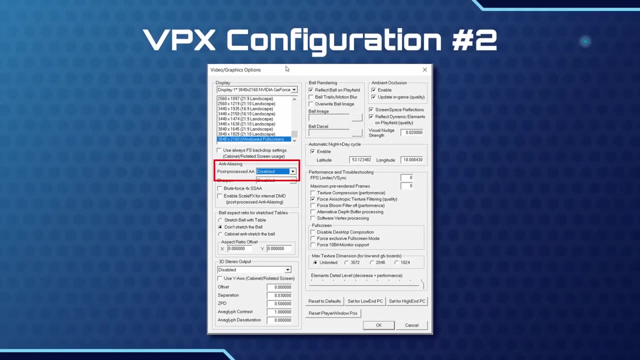 The anti-aliasing is enabled with the quality SMAA setting. Ambient occlusion is enabled, Screen space reflection is enabled And reflect dynamic elements on playfeed is enabled as well. Second configuration is the same as the first one, but the anti-aliasing is disabled. 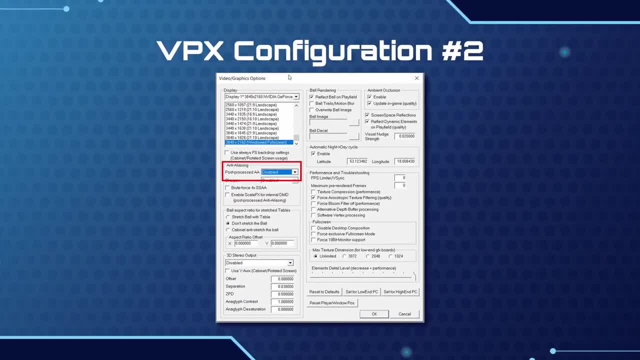 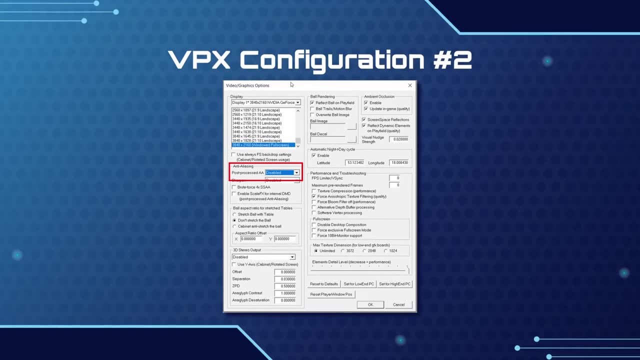 In my opinion, the AA is not even needed on the 4K screen and I don't use it, but some of you may be interested to see the performance difference using it and not using it at all. Insert configuration compared to the second one. 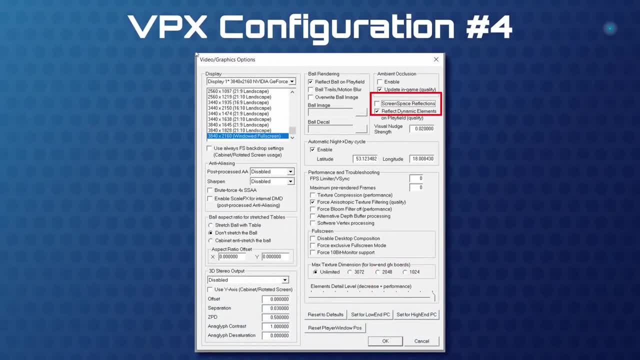 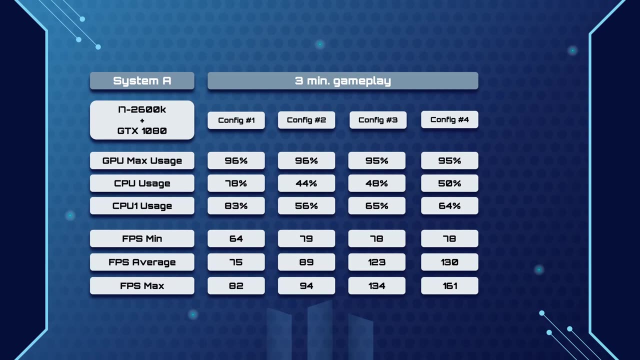 Ambient occlusion is disabled And the last one also has the screen space reflections disabled. For the performance recording I have used the MSI Afterburner and RivaTuner statistics server Test on system A I7 2600K with GTX 1080. after 3 minutes of gameplay on each of those, 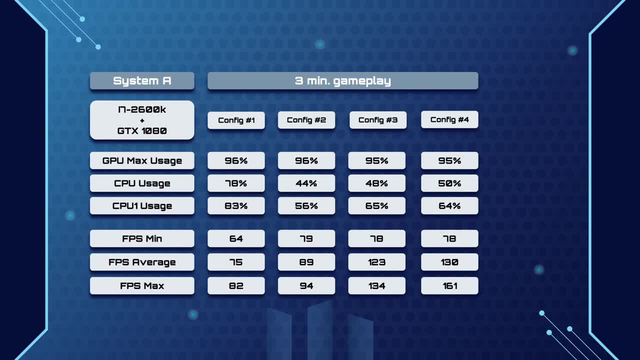 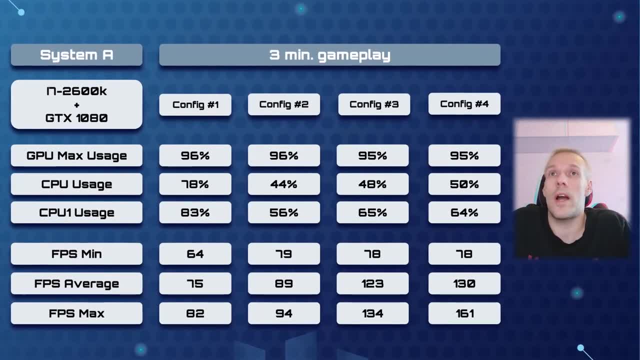 four configurations shows the following results. As you can see, I should be safe with those framerates, Looking at the minimum FPS, Which shows how low framerate dropped during multiball and when many flashing lights were kicking in, Even at the configuration number 1, which is the most demanding because of the AA use. 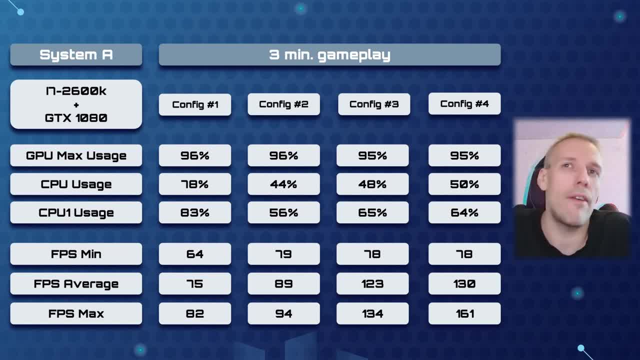 the minimum is above 60 FPS, and that should be enough for me playing VPX on the 60Hz 4K screen, But unfortunately the usage of the CPU is high, so the drop can not only happen from the VPX itself. 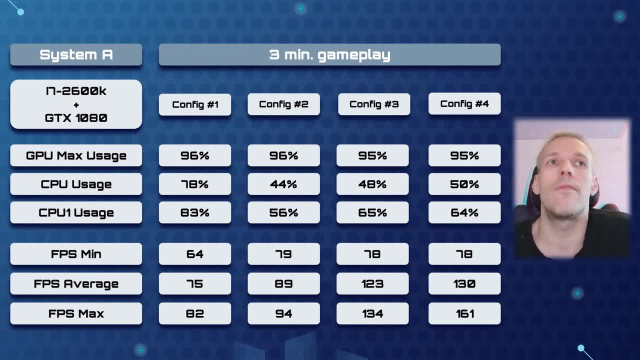 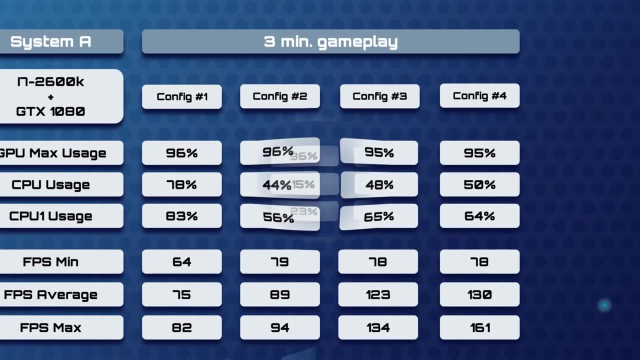 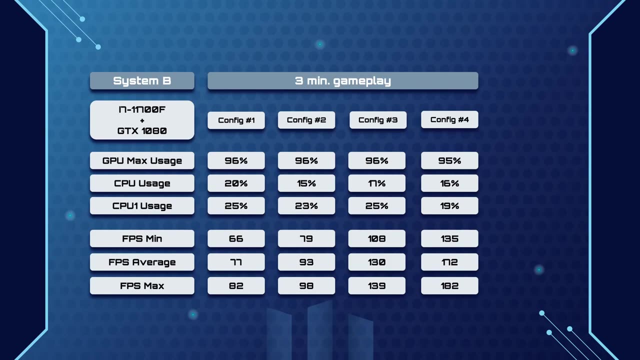 But from other things like DMD backless and from Windows system itself too. In fact, only config 3 and 4 was giving me the gameplay. that had stuttering or hiccups on very low level, But unfortunately they happened. Let's see now the result of the gameplay after changing CPU to 11th gen i7 11700F. 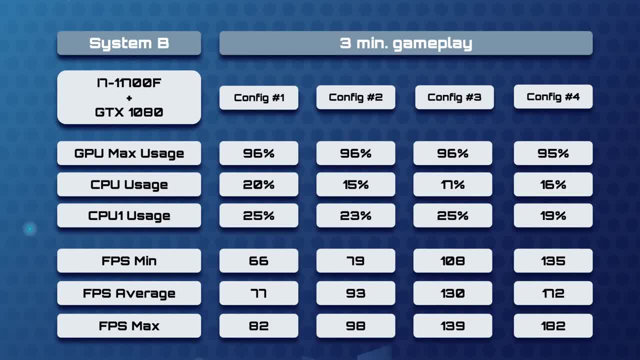 On configuration 1 and 2, there was no huge difference In terms of the performance. In terms of framerate, it was lower than 5% FPS gain. But the configuration 3 and 4 changed things significantly in terms of the lowest and average. 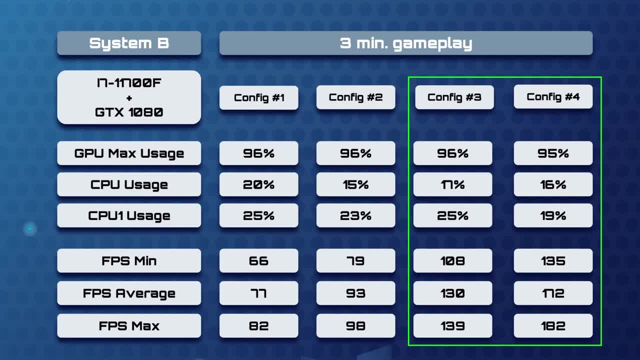 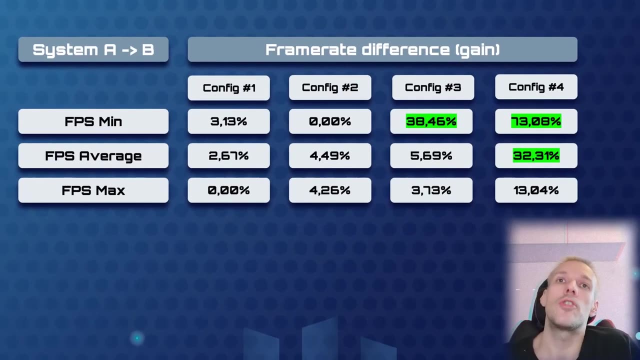 framerate achieved. What is important besides the framerate here, in my opinion, is the CPU usage now sitting around 20-25%, while with older CPU it was around 80% at configuration 1 and around 50% at configuration 2.. Here are the percentage framerate changes on each of the configuration from old CPU: 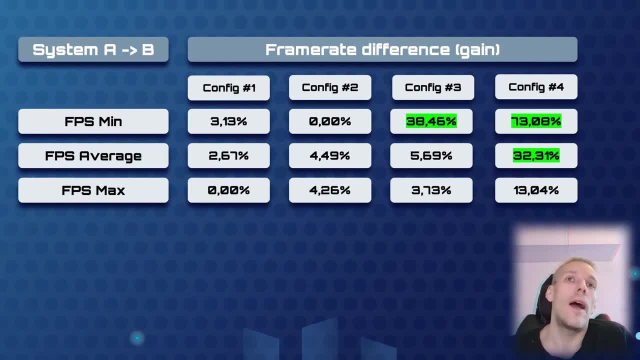 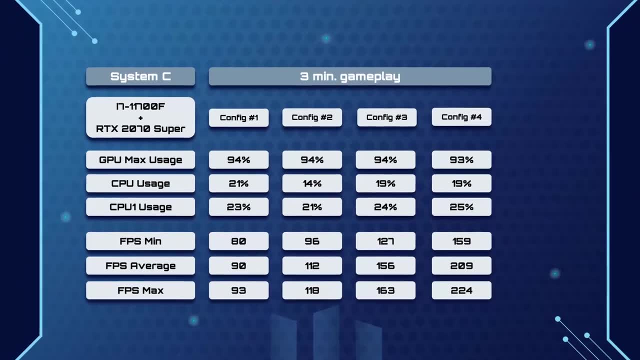 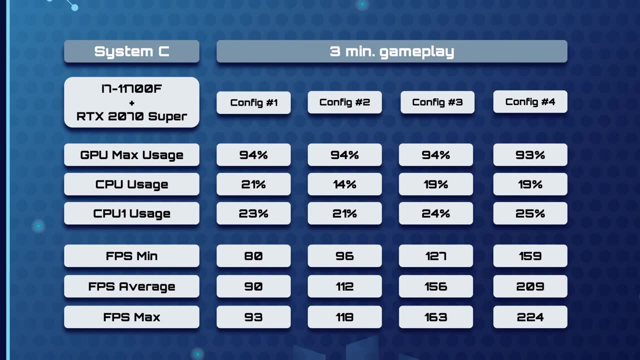 to new CPU system with GTX 1080.. Highest difference noticed in the config 3 and 4 market with the green color. Now let's look at the same new CPU with the better graphics card, RTX 2007 super. The framerate difference in percent is 80%. 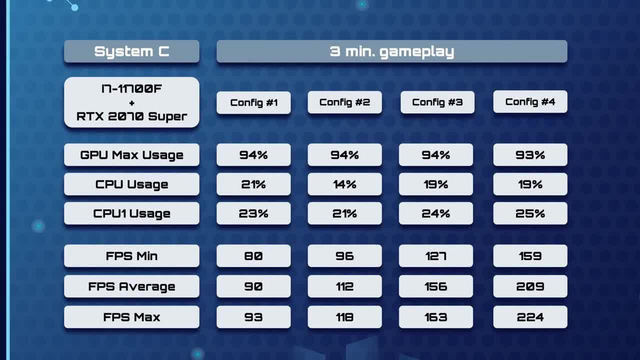 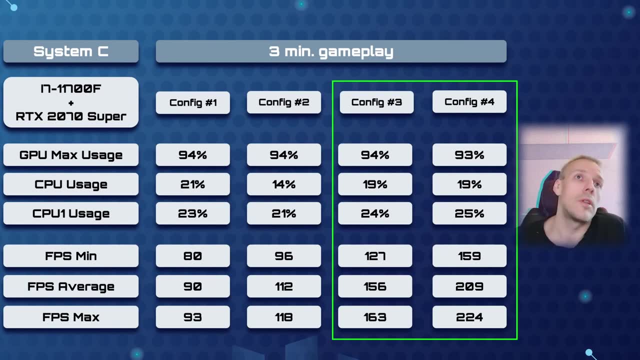 It's averaging around 20%, which is how the internet benchmark computing power of the RTX 2070 super over the 1080 is expected to be. Looking closer to a configuration 3 and 4, I see a lot of potential which can be utilized. 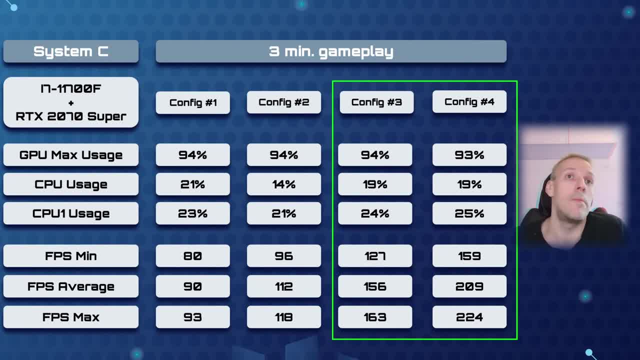 even with the 120Hz monitor or maybe even 144Hz one, With the configuration 4 in mind, Average of 200Hz, Average of 200Hz, Average of 200Hz, Average of 209 frames per second in configuration 4 is very promising. 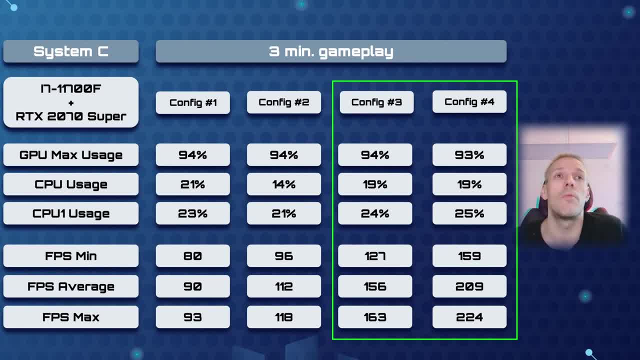 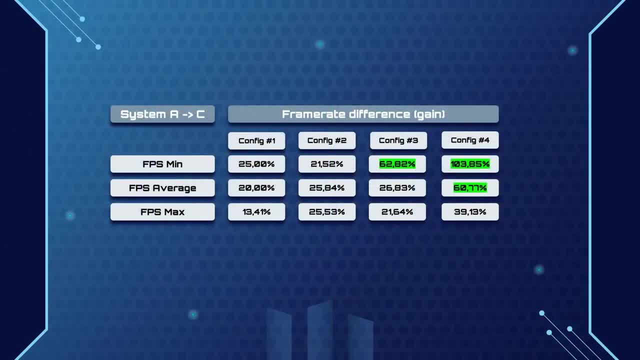 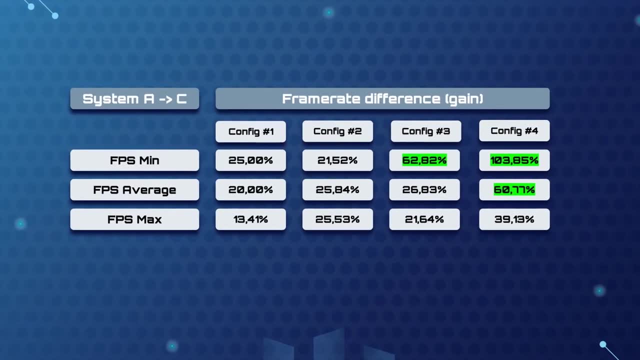 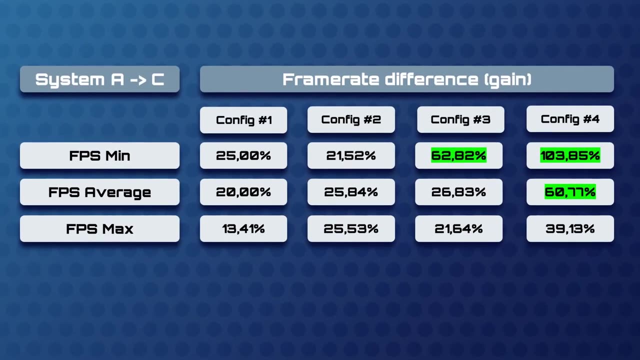 Maybe in the future I will get a 120Hz monitor to get more fluent gameplay and less lag. That would be nice. Final result of the change from i7 2600K with GTX 1080 to the i7 11700F with RTX 2070 super. 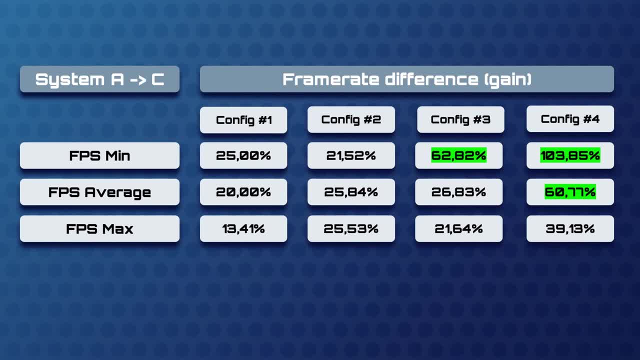 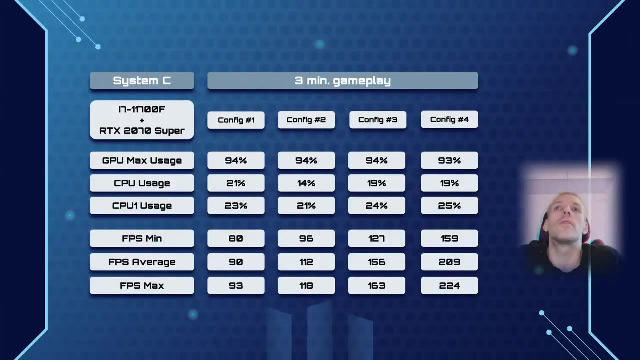 is significant, especially in the configuration 4, with over 1% framerate gain for minimum value- The value that happens when heavy light or multiple kicks in- And 60% gain for the average FPS value, Taking into consideration that the average FPS is the most common and the minimum only. 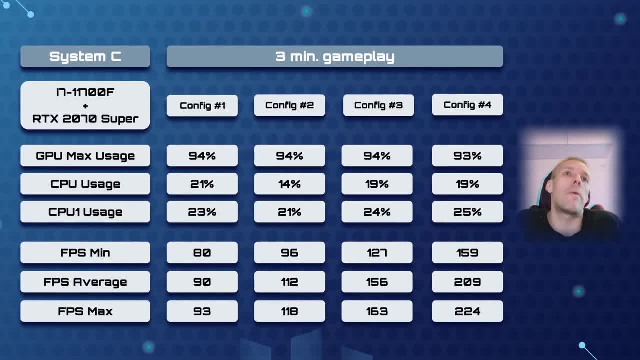 happens sometimes during drops. I can assume that the best monitor to be used for this setup would be 120Hz. That's it. That's it, One with some kind of variable refresh rate technology applied, Not taking the TV into consideration, because TVs doesn't have the display port and are 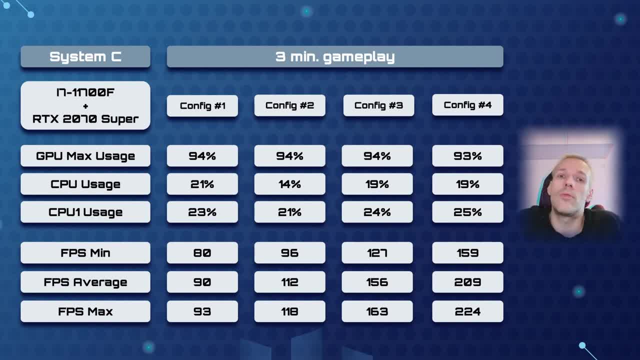 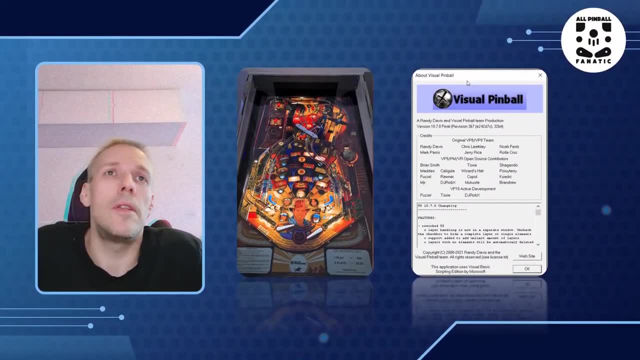 using HDMI 2.1, which RTX 2070 is not equipped with. For the TV with HDMI 2.1, the RTX 3000 series card is needed, unfortunately. I did one more test while playing the same Indiana Jones, But running it with pinup popper and using exclusive fullscreen mode, and the results. 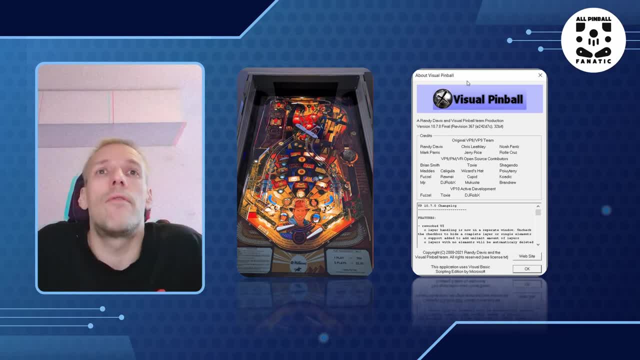 were almost the same for all the configurations, From VPX alone in windowed mode to pinup popper in exclusive fullscreen mode, gives 6-8% frame boost. But what is important here, in my opinion? the pinup popper with all those screens and 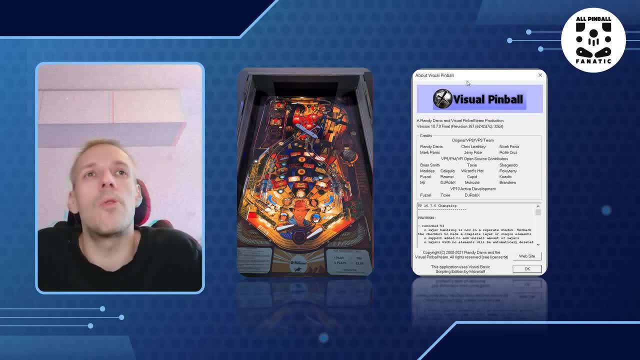 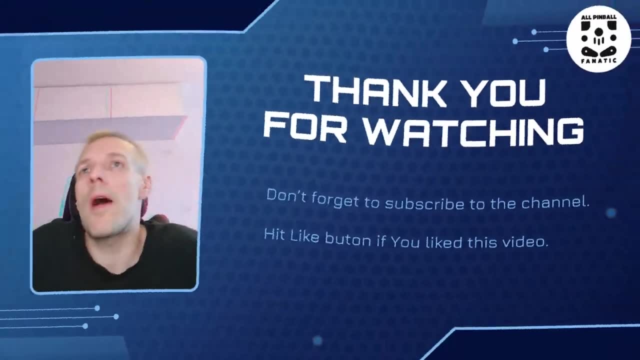 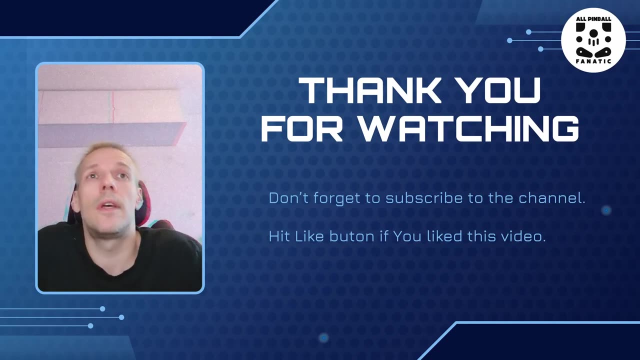 videos playing along with the table can eat a lot of space. So to sum up at this point, I'm super happy with the CPU motherboard and graphic card change I did. The gameplay is now super fluent and I don't see any stuttering or dropped frames. I also need to mention that the hardware change was really easy with the Windows 10, which was a real surprise. I didn't have to do a fresh Windows installation, I just ran the disk on the new CPU mobile RAM system And Windows did all to properly switch from the old one to the new one. 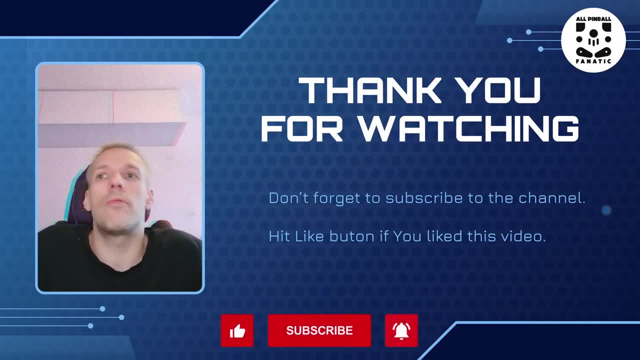 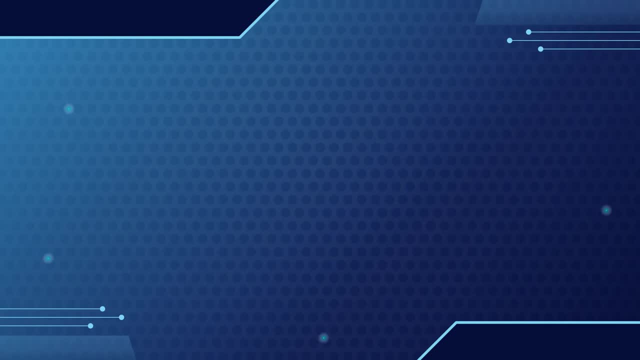 Thank you for watching this video. I hope that you found it interesting. don't forget to subscribe to my channel. Happy flipping and see you next time. Thanks for watching. See you next time. Bye.